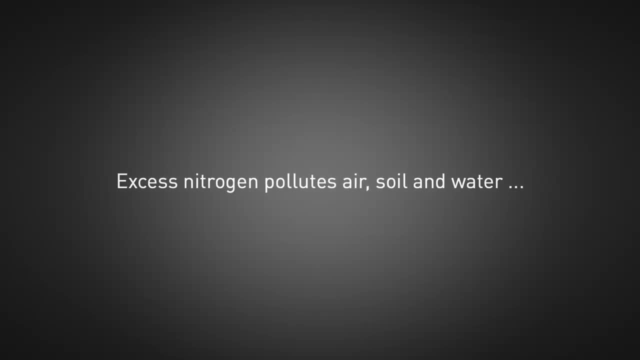 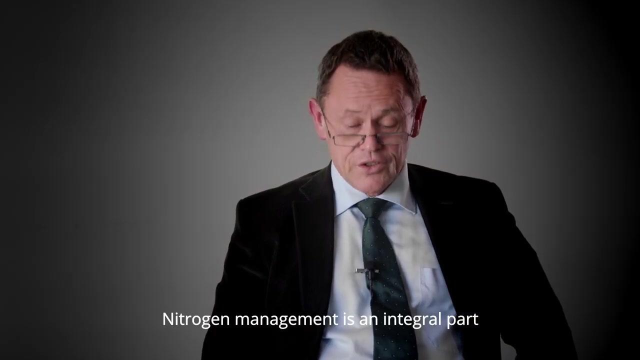 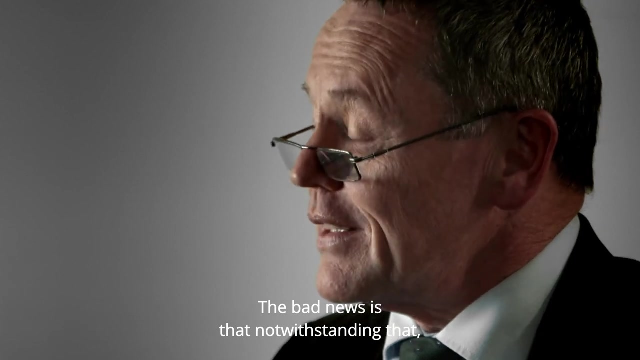 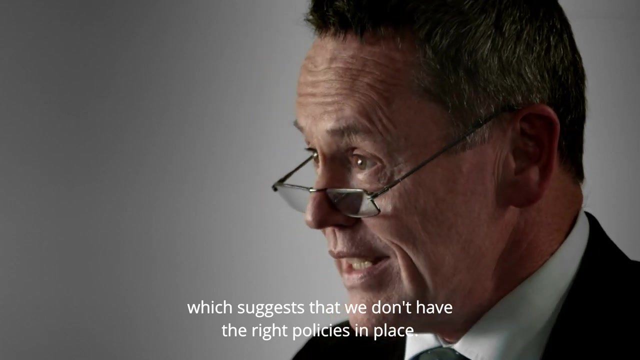 on the environment that have been overlooked. The good news is that we're not starting completely from scratch. Nitrogen management is an integral part of environmental policies in quite a lot of countries. The bad news, however, is that, notwithstanding that, nitrogen pollution is, in many cases, getting worse, which suggests that we don't have the right policies in place. 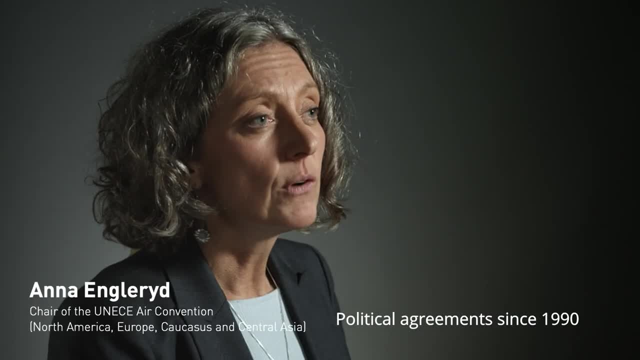 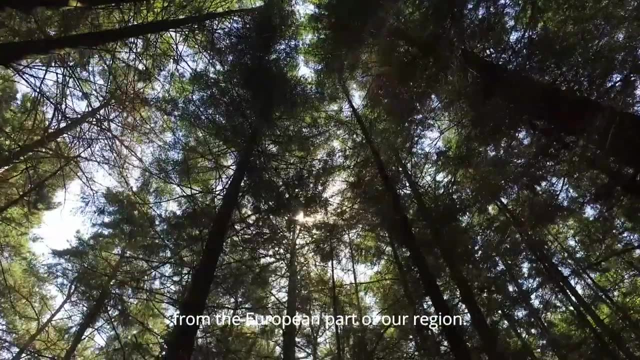 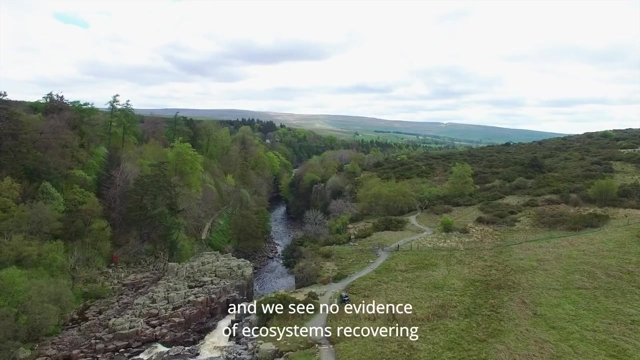 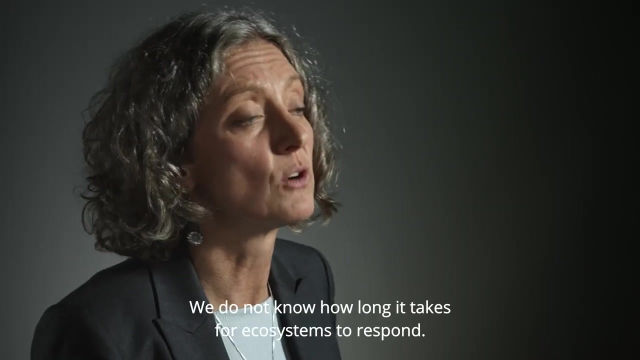 Nitrogen is a major challenge to us Political agreements. since 1990 has substantially reduced nitrogen oxide emissions from the European part of our region, But we still see critical loads of nitrogen deposition being exceeded in large parts and we see no evidence of ecosystems recovering where the deposition has been reduced. We do not know how long it takes for ecosystems to 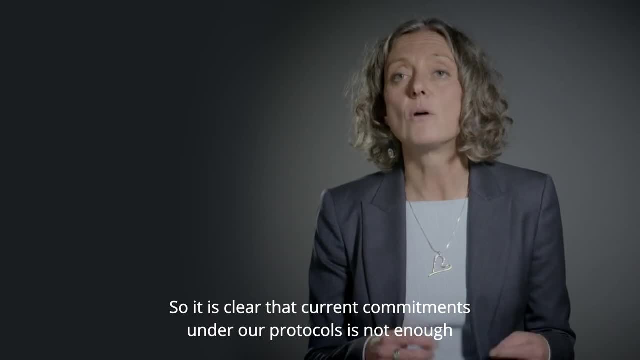 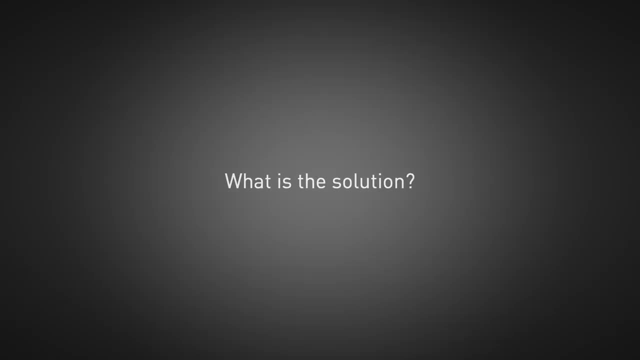 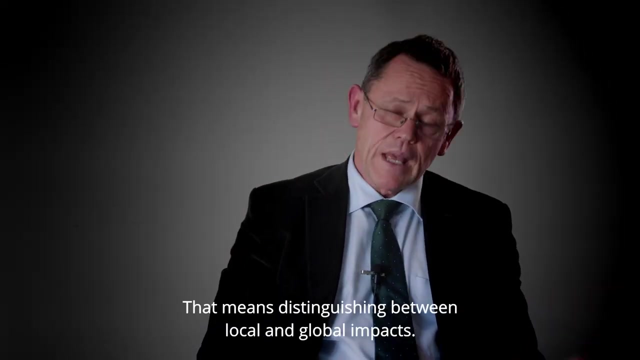 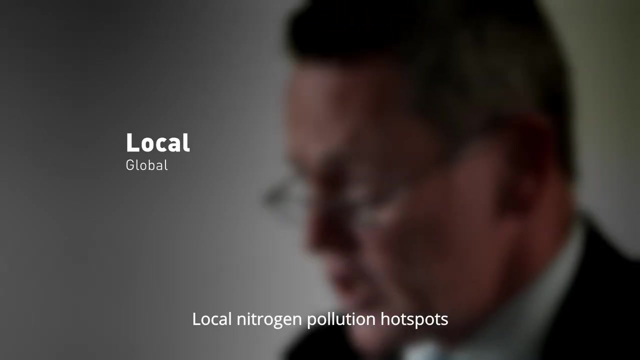 respond. So it is clear that current commitments under our protocols is not enough to hamper further accumulation of nitrogen in the ecosystems. That depends on where the pollution is taking place and the form it takes, and that means pushing between local and global impacts. Local nitrogen pollution hotspots will require a cap. 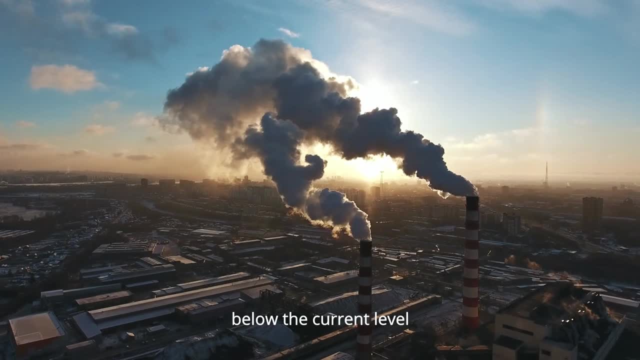 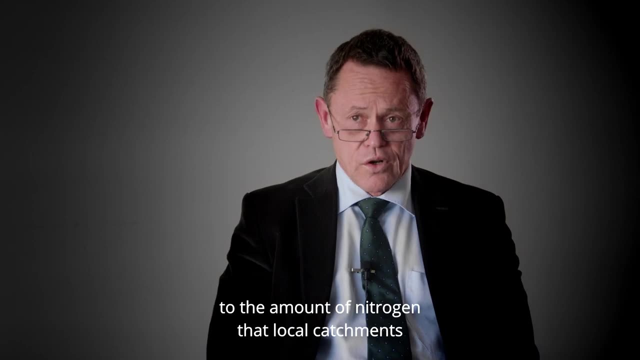 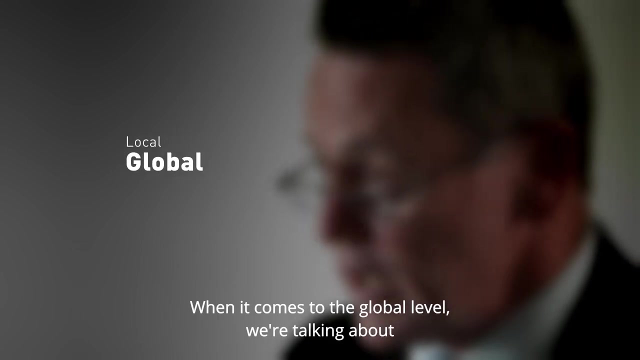 They'll actually require a reduction below the current level if we are going to avoid permanently damaging ecosystems. There are limits to the amount of nitrogen that local catchments can absorb without causing permanent harm. When it comes to the global level, we're talking about the 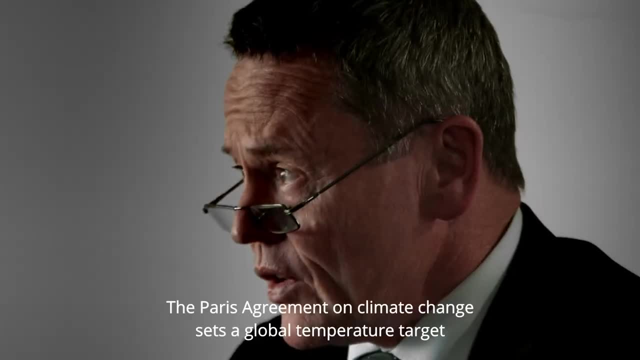 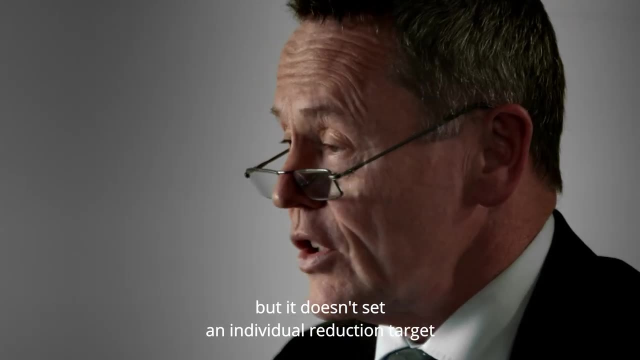 climate change implications of nitrogen. We're talking about the climate change implications of nitrogen, Nitrous oxide. The Paris agreement on climate change sets a global temperature target, but it doesn't set an individual reduction target for each of the greenhouse gases. That's been left. 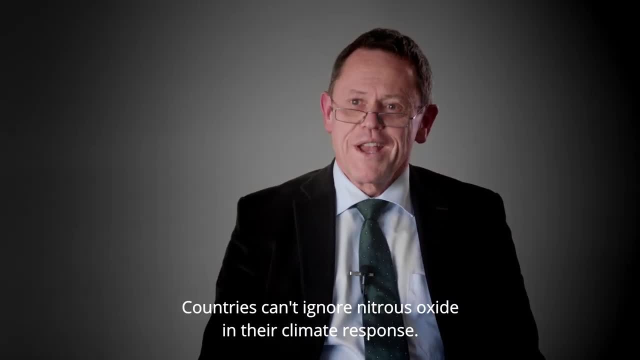 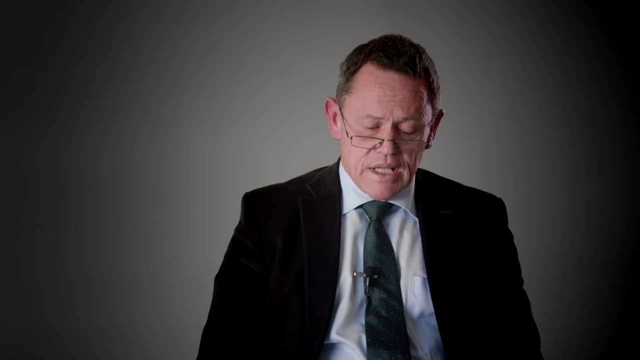 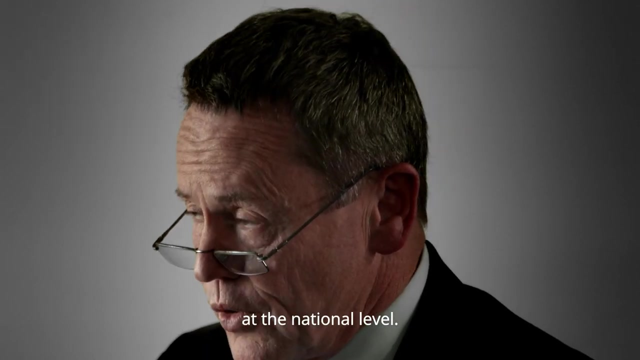 up to countries to do. Countries can't ignore nitrous oxide in their climate response. We need to monitor and report progress on tackling nitrogen pollution at the national level. According to the last protocol, the Gothenburg Protocol parties have committed to establish.